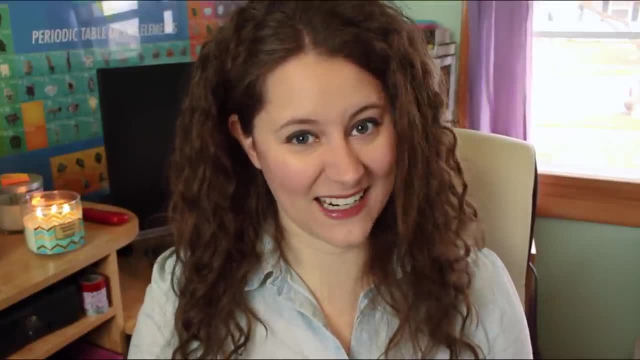 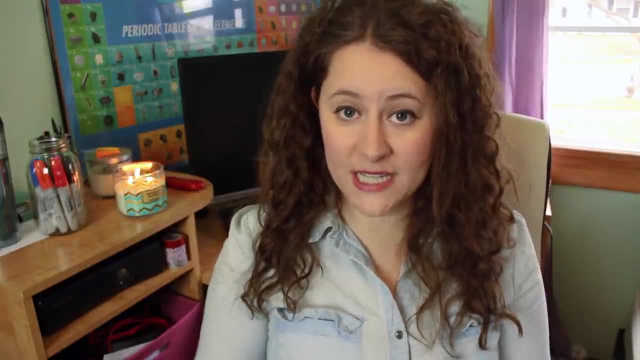 This way, we can have a discussion about them much more easily. It's going to be fascinating. Let's start with a term that is probably familiar to most of us: the epicenter of an earthquake, Let's say. you're looking down on the earth from bird's eye view. This is also called map view. 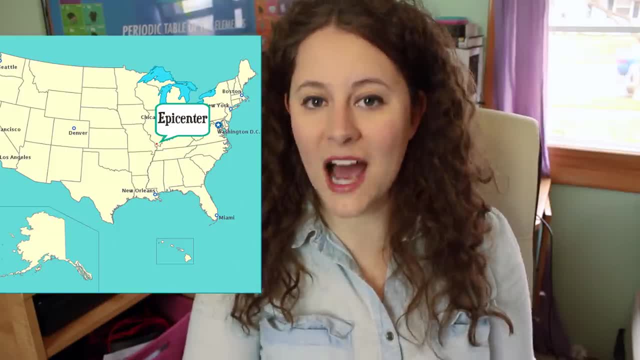 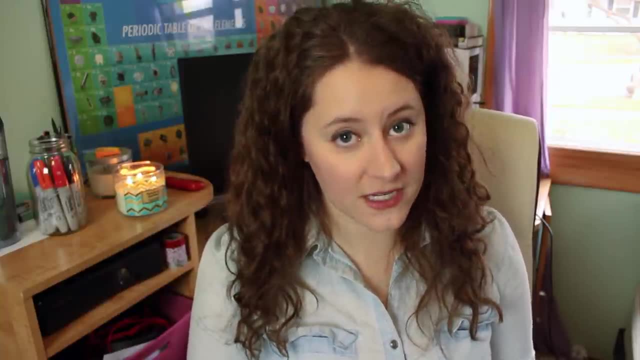 It's what the map is. It's map view. The epicenter is the point on the map where the earthquake occurred. However, if you were to look at the ground in 3D space, the epicenter would just be a point on the surface. 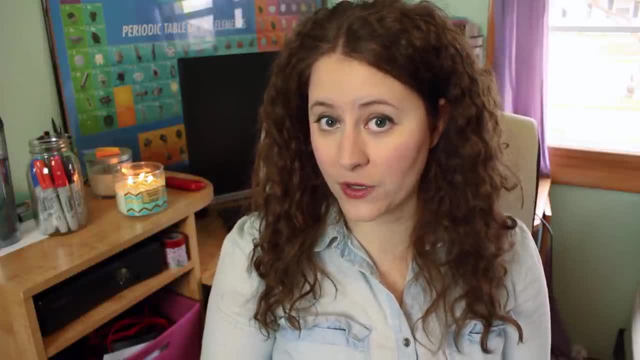 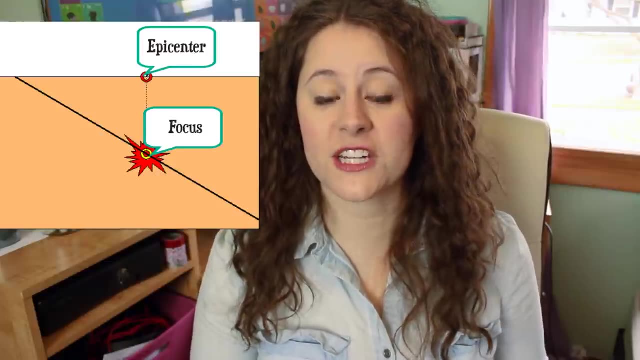 Earthquakes don't typically happen on the surface. they happen underground. The point in a 3D view of the earth where the earthquake actually happened is called the focus. When an earthquake occurs, the characteristic shaking is actually caused by seismic waves. 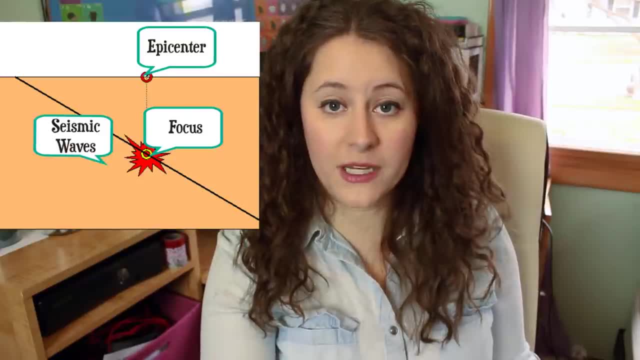 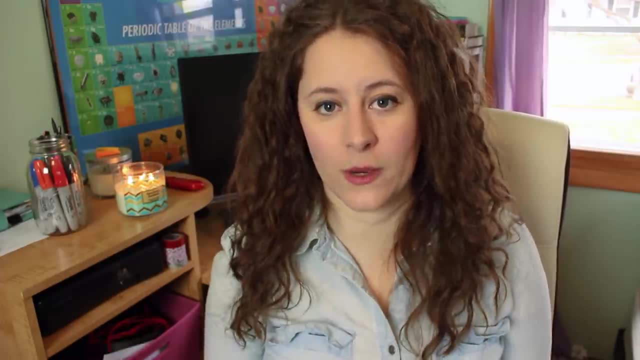 These seismic waves radiate out from the focus. So in 3D we have a focus, In map view we have an epicenter, And seismic waves are what cause the earthquake. So what exactly is an earthquake? We all know that it is a shaking of the earth and is also sometimes called a tremor or a terror. 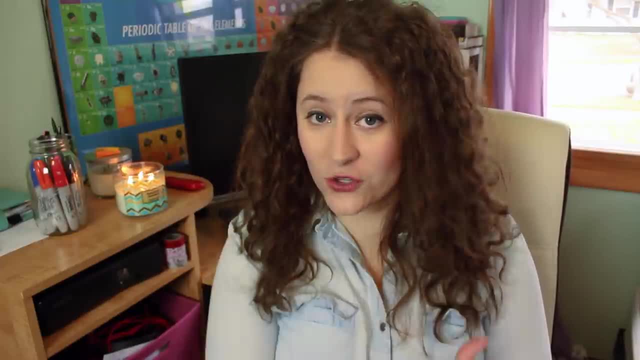 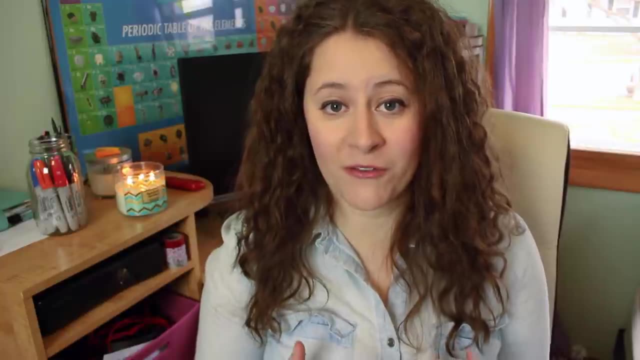 What causes this shaking is the movement of rock against one another. Two rigid pieces of rock trying to move up against one another does not happen nicely. The rocks fight this movement, which causes a buildup of rock against one another. Eventually, the pressure gets to a breaking point. 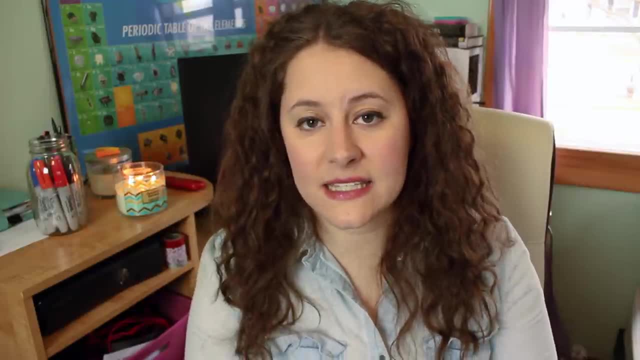 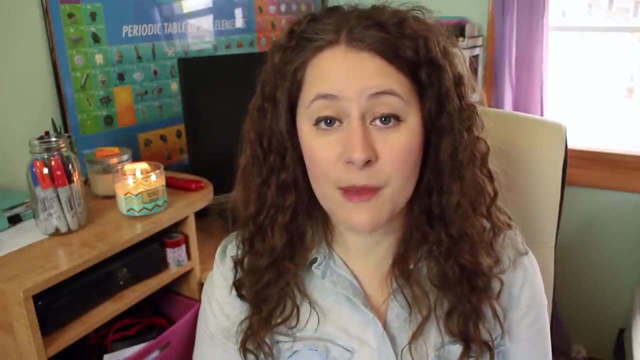 at which time the rocks give way and slip. That slip is what releases the seismic energy and results in the shaking. Now that we know specifically what an earthquake is, where do they occur? Because earthquakes are caused by moving rock plate, boundaries are ripe with earthquake opportunities. 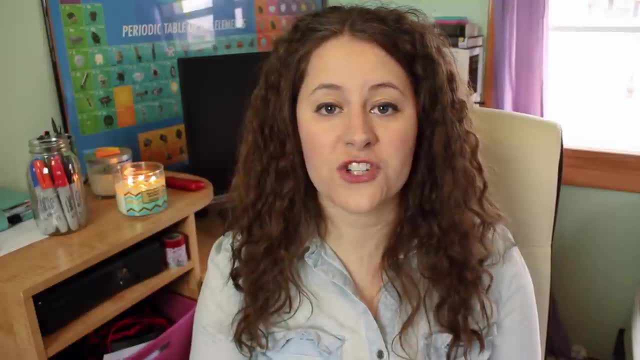 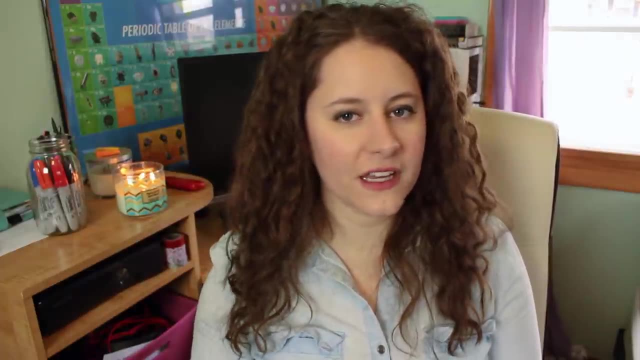 Lithospheric plates cover the earth much like a shell Plate. boundaries are locations where several different pieces of this rock meet and are interacting. These interactions are what cause most of the earthquakes in the world. Now, I know what you're thinking, But I live in XYZ time. 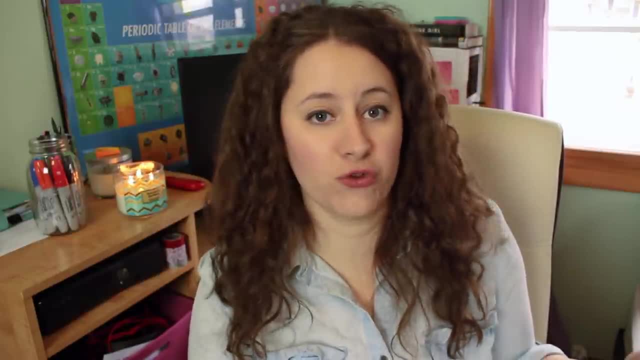 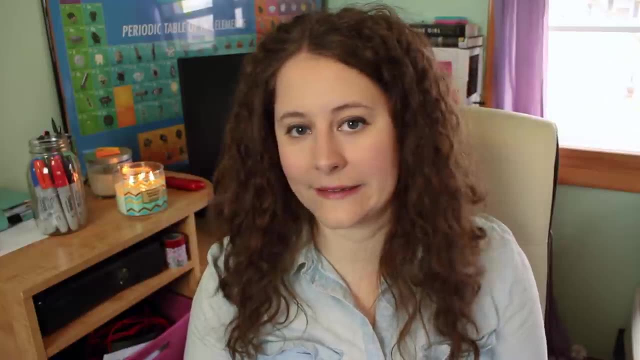 And we are in the middle of a continent, not next to a plate boundary, and we had an earthquake last week- And that's because you can get earthquakes wherever there are faults, And there happen to be faults all over the continent. In fact, one of the most famous areas for interplate earthquake activity 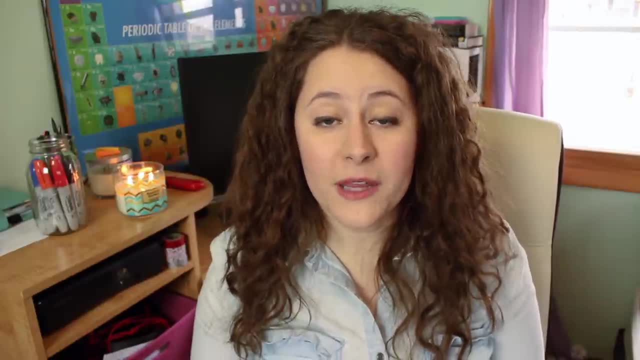 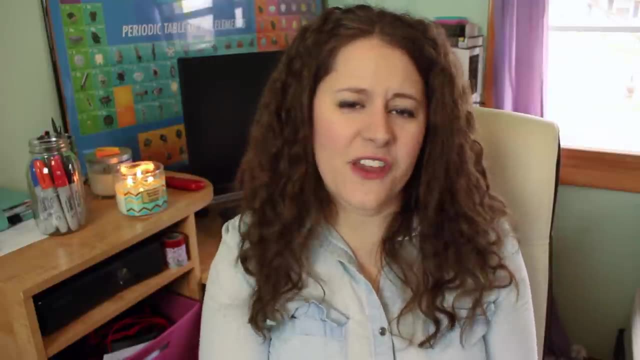 is the New Madrid Zone in my home state of Illinois. So while interplate earthquakes are more rare, they definitely do happen. The USGS records about 50 earthquakes a day But, Jessica, I don't feel and or hear about earthquakes every day. That's because most are too small to be perceptible by humans. Wonder what that cutoff is. Stay tuned for later in the series where we will discuss how we measure earthquakes, types of seismic activity, effects of earthquakes and the geomythology of this phenomenon.